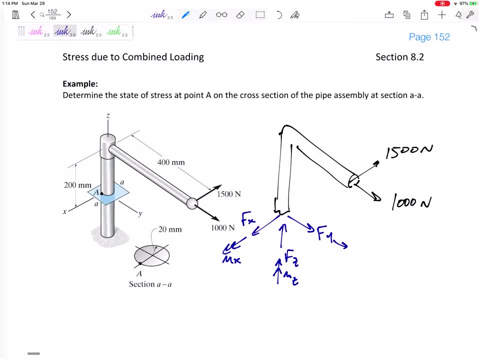 a double arrow MX, a double arrow MY. but you know that the direction of the moment is really the axis that the moment is rotating about, right. Remember, for 2D problems all of our moments were in the K direction because clockwise and counterclockwise on a 2D sheet of paper would. 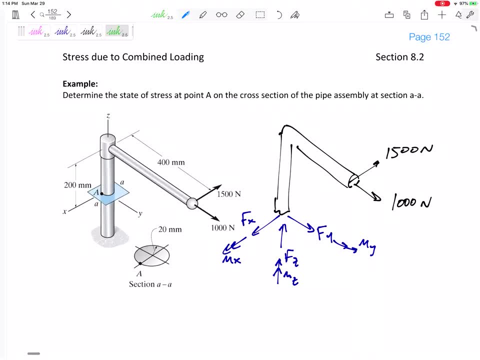 mean it's rotating about the Z axis, you know, out of the page or into the page. So, using the right-hand rule and curling my four fingers in the direction of the moment, the direction of the rotation, my thumb is the- you know the axis that the moment is rotating about. So, using the, 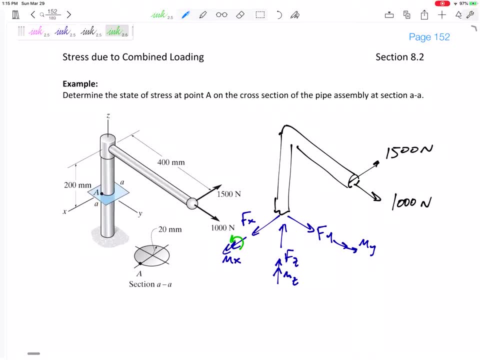 right-hand rule. let's think about this: MY, This, MY, my fingers, my four fingers would be curled in that green arrow, right In my right hand, my three fingers would be curled in that green arrow, and so my thumb is pointed in the X direction. Here the 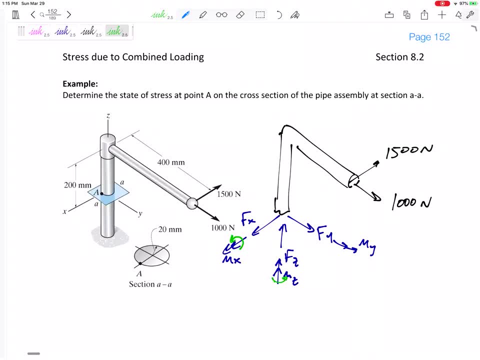 MZ. oops, sorry, let me do that at the moment. MZ, my three fingers are curled that way. My thumb is pointed up. MY, my four fingers are curled that way. My thumb is pointing in the Y direction. 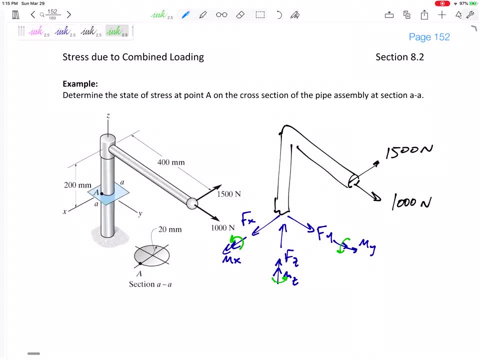 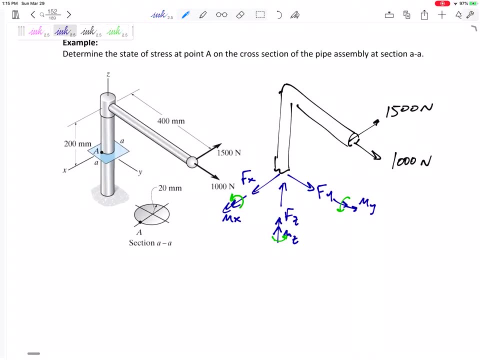 All right, we need to really be able to understand those moments, their directions. Okay, so let's solve for these three internal forces and three internal moments. Well, it's really six unknowns, but we have six equations. We can sum the forces in: X equals zero. 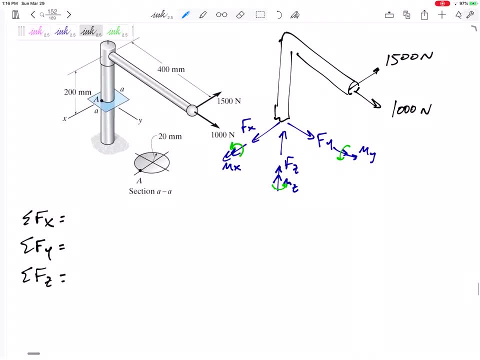 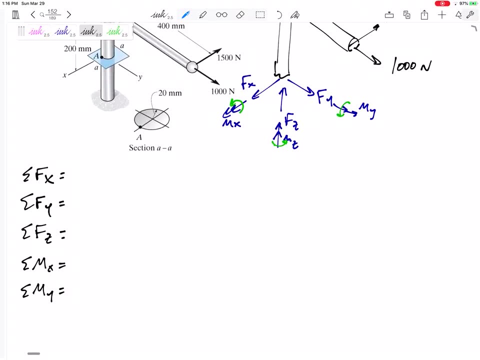 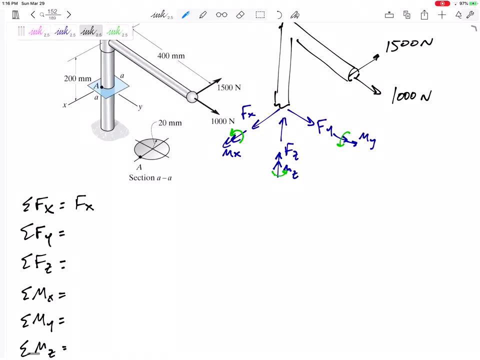 some of the forces in Y equals zero, some of the forces in Z equals zero. We can also sum: the moments about the X axis equals zero, the sum of the moments about the Y equals zero, the sum of the moments about the Z equals zero. And so I have my internal FX in the positive X direction, my 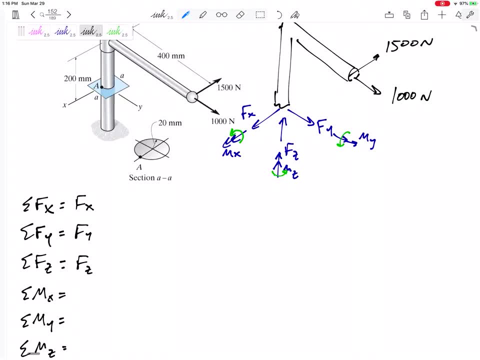 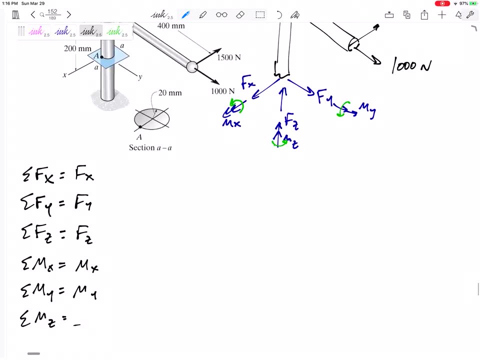 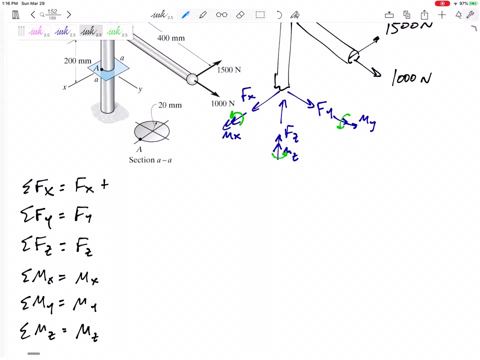 internal FY: I drew that in the positive Y direction. my internal FZ: I drew those in the positive axes. my internal MX, MY MZ, All right, so those are my internal ones, but then all of the external ones are going to sum. 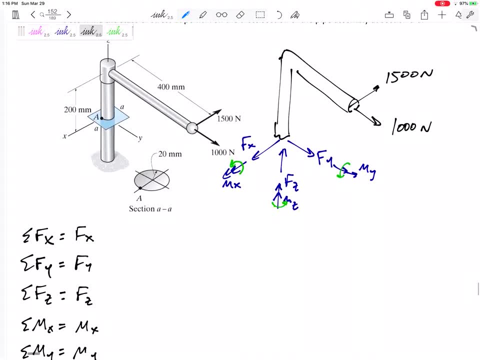 to zero. I'm the internal plus external sum to zero. What do I have in the X direction? Let's see, I've got that 1500, but it's in the negative X direction And I've got the thousand that is in. 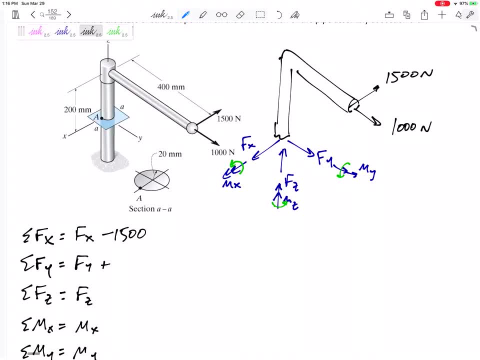 the positive Y direction. Oops, positive Y direction. Those are the only forces I have, So I guess my force equations are done. I can sum those equal to zero, And what would I get? FX, be careful. sum them equal to zero, And so the math would. 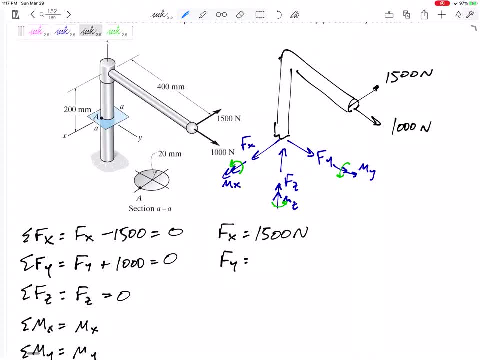 come out to be positive: 1500, FY negative: a thousand, FZ zero, All right, so maybe I shouldn't box that in. That's not my final answer, but that's a very important part of your answer: getting that the internal forces are. 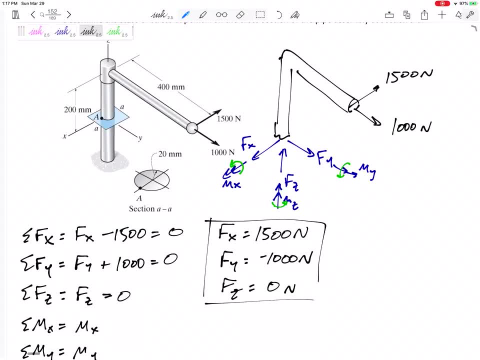 1500 in the X, negative thousand in the Y and zero in the Z. Now I do that by summing the forces equal to zero. You could also just kind of ask yourself: okay, what do I need internally to counteract the external forces? right, This is in static equilibrium, It's going to add up to zero. 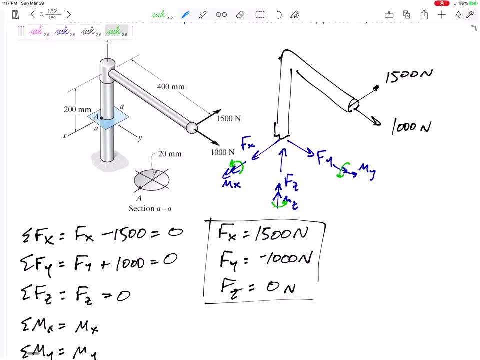 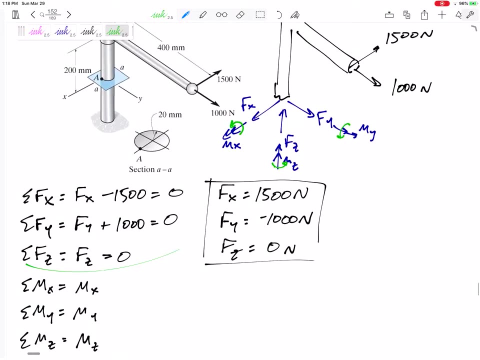 And so you can think about them adding to zero, or you can think about them just counteracting the external. The internal ones counteract the external ones. Does it make sense that we need a positive 1500? Negative, 1000 in the Z, a zero in the Z, sorry, Okay, so this is my process, You might. 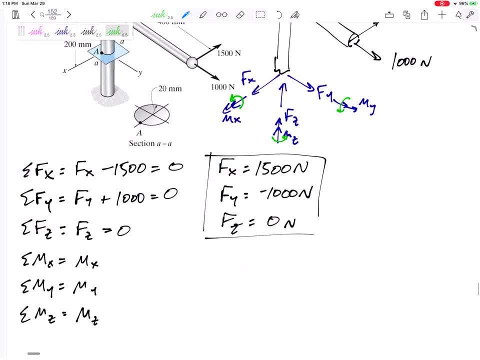 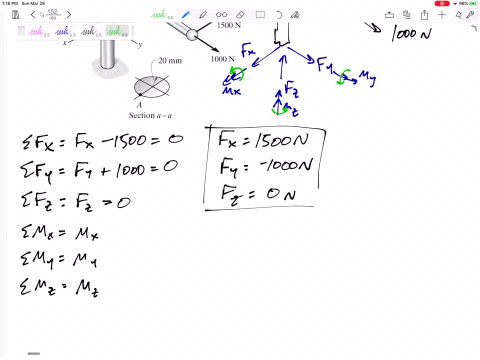 could jump straight to that, the more comfortable you are with these All. right now, the moments I don't think I'm going to be able to jump straight to. okay, what are the internal moments that I need? I think you really need to sum the moments in: X equals zero. sum the moments. 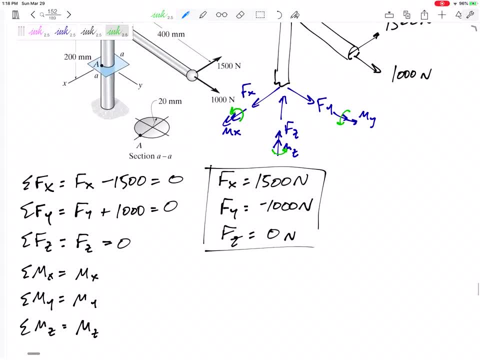 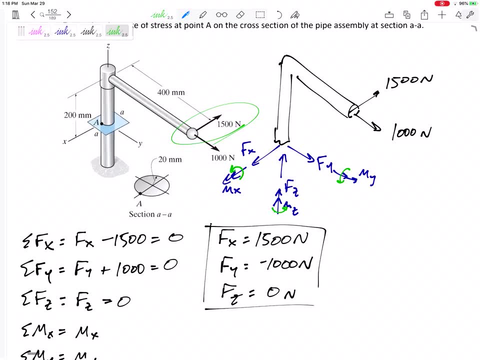 in Y equals zero. sum the moments in Z equals zero. Okay, the way I like to think about it is: every force, every force can create two moments. Every force that is in a that is fully in one direction can create two moments in the other two directions, depending on how it is offset from the cut. 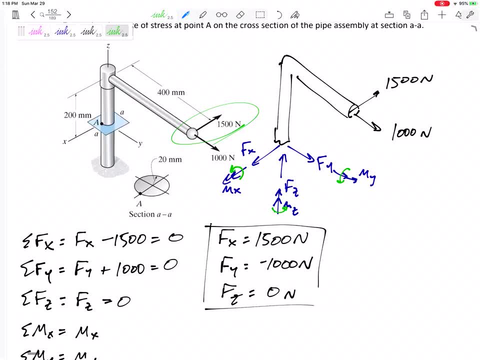 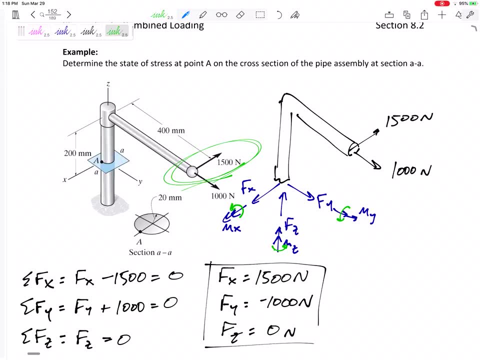 All right. so we are looking at what type of moment will this 1500 Newton force create about the cut? There might be two. Do you? which one do you see First? the one that I see first is if I'm going to be pushing this way right here on this arm. 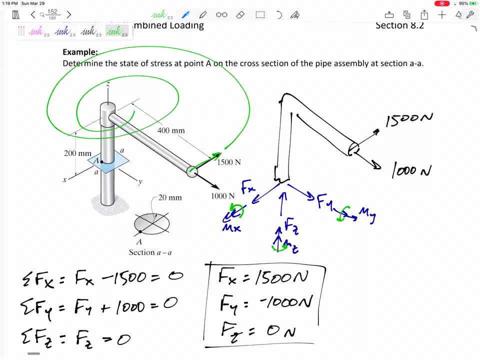 I'm going to create this rotation about the Z axis. See that If I am got a force of 1500 Newtons and a moment arm of 400, that would create a rotation in the Z axis. So I'm going to come. 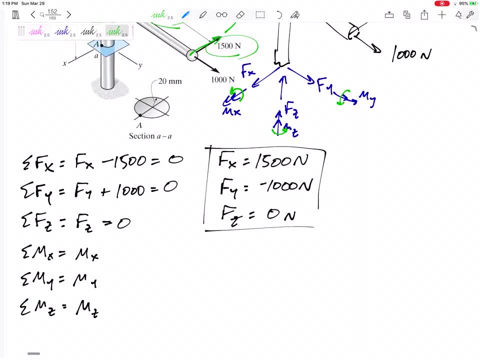 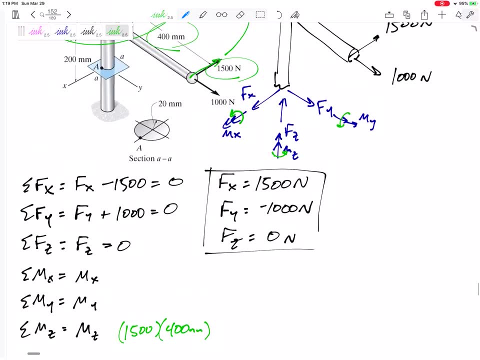 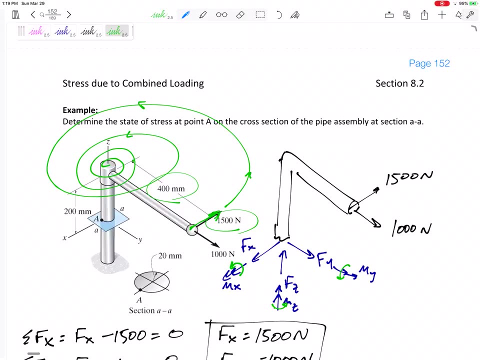 down to my Z equation. Now I'm going to say, okay, uh, 1500 Newton's Acting 400 mm away, a positive or negative Z, if, if it's this way, If this is my arrow, you know what type of rotation does this cause? just what? use your right hand, curl it about Z. 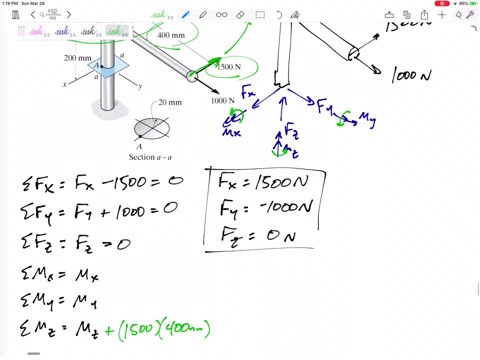 My thumb is pointing in the positive Z, So that would be a positive moment. Let's double check that, And we did that a couple of times. Let's double check that, And we did this a while ago, but't attempt to repeat. Let's double check that, And we'll do that a couple of times. let's double check that, And we did this a while ago, but't attempt to repeat. Let's double check that, And we did this a while ago. 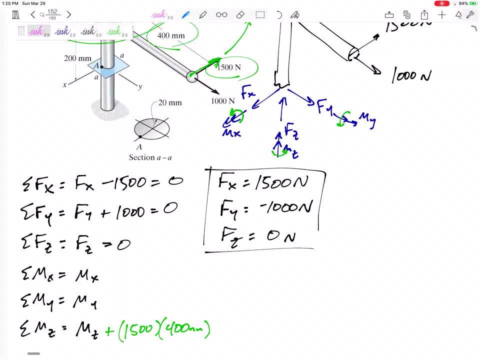 this a long time ago, didn't we? second week of class or something? so it's been a while. I got it, got to review, got to visualize these moments. this 1500 is in the X direction and that moment arm is in the Y direction, so it makes sense it. 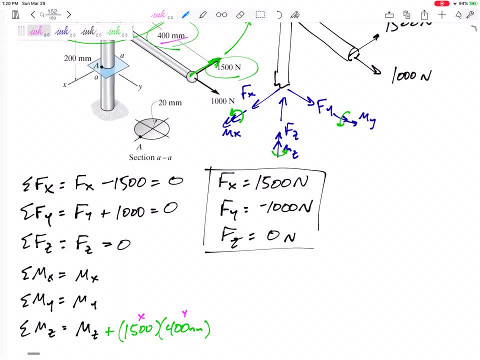 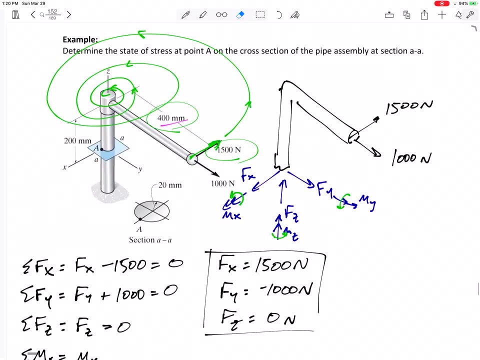 would create a Z moment. right, an X force with a Y moment arm would create a Z moment. remember that the moment is perpendicular to both the force and the moment arm. so that's a good way to double-check, right there now, the positive, negative. I just visualize. you just have to visualize it now, if you. 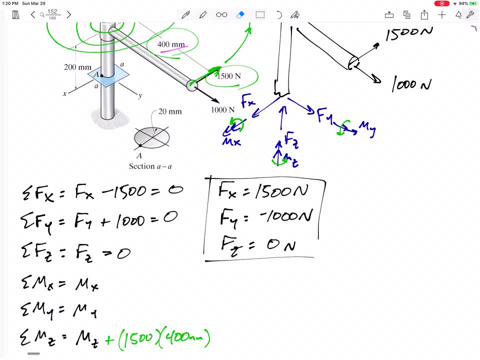 really want to. maybe someone will do this, maybe I'll do this, I don't know. there's a formula for whether a this would be a negative X with a, you know, positive Y moment arm. would that create a positive or negative Z? and it really goes back to the cross product moment is. 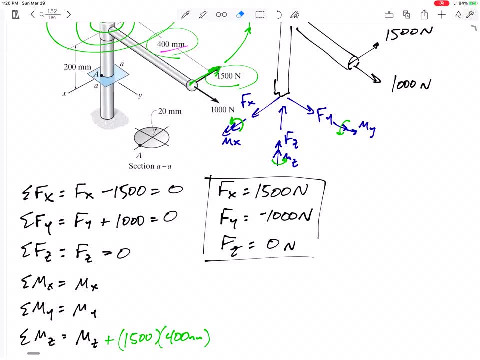 you know, if you have a negative X with a positive Y moment arm, would that create a positive or negative Z? and it really goes back to the cross product moment. is R cross F? right? it's not F cross R, is it? y'all double-check me on this, right R? 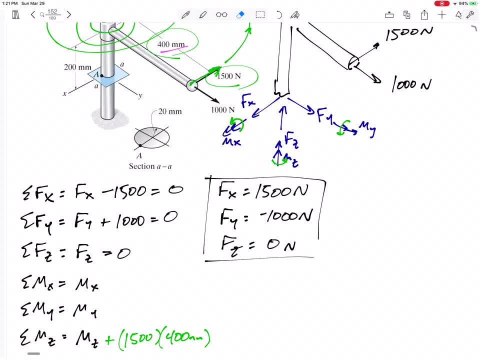 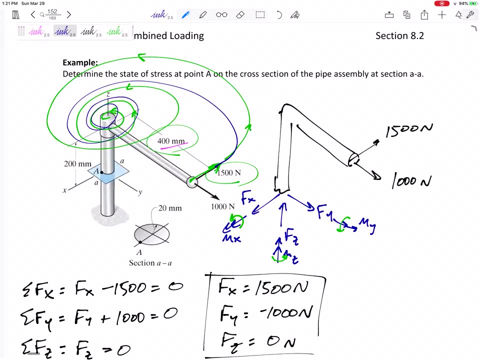 cross F and so you can really go back to like doing a cross product of the R cross with the F. I don't know, I just can visualize and hope you can visualize right, that this would create a positive right-hand rule, positive rotation about the z-axis: okay, but it could. 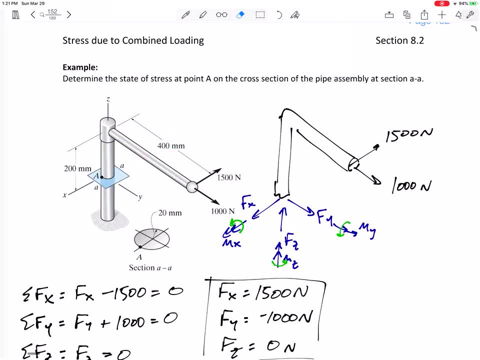 create another moment. it could create another rotation, depending on how it is offset. do you see that it is also offset? it's 200 millimeters above the cut. it's 200 millimeters above the cut and so, if I am pushing with some force, 200. 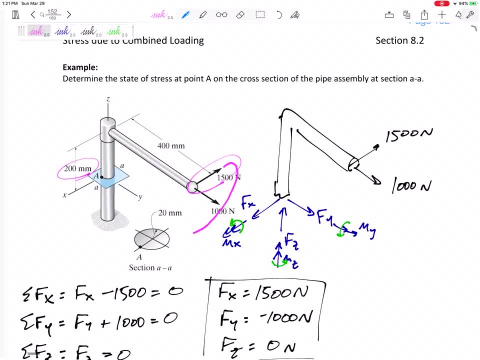 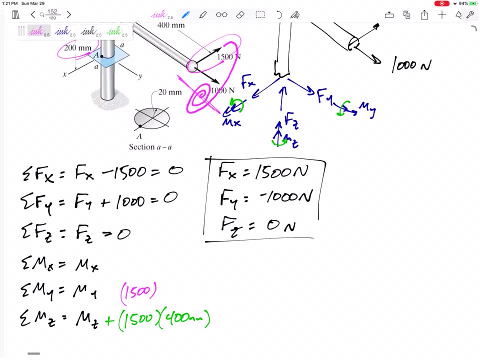 millimeters above the cut. it can curl down here and it can rotate in the about the y-axis, rotate about the y-axis. so 1500- I'll do this in pink. 1500 with a 200 millimeter moment arm would create a why rotation. 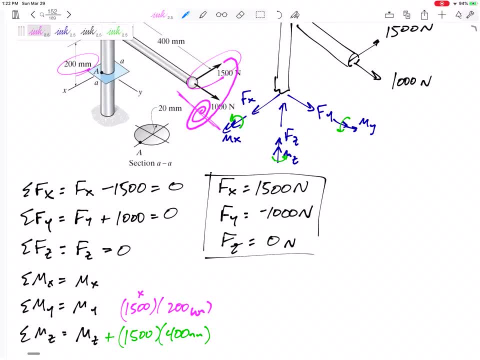 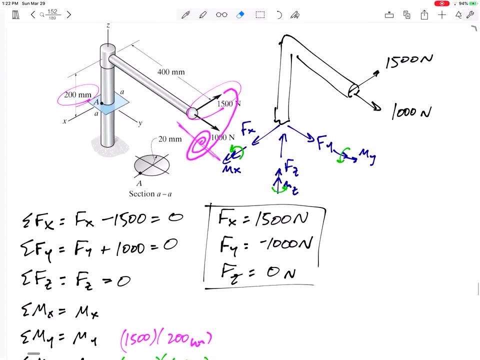 this is in the x-direction, this 200 is in the z. so yeah, it makes sense that it would be a y moment at X force with a Z moment arm. we created y moment, positive or negative. all right, that rotation that I just drew circling around, I'm going. 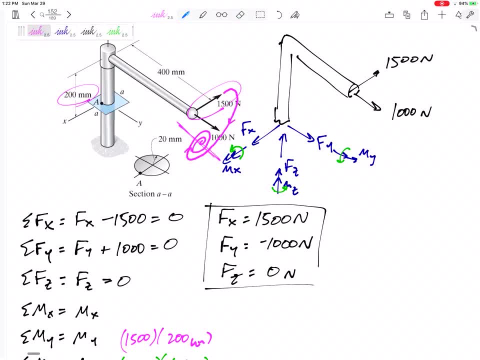 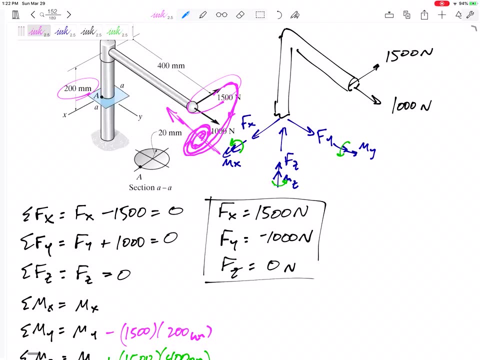 this way, this way. this is straight. if, when I'm your, so here's my haciendo this way, this way, If I'm rotating about here to here, to here to here, using my right hand, curling my fingers, my thumb is pointed this way in the negative y, So 1,500 newtons times 200. 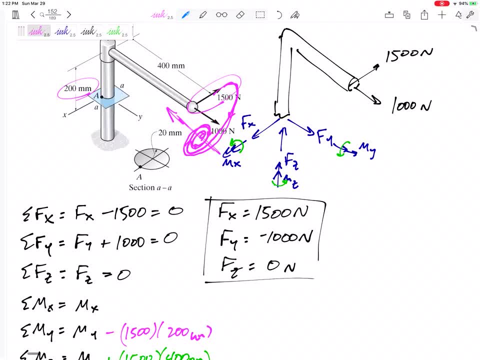 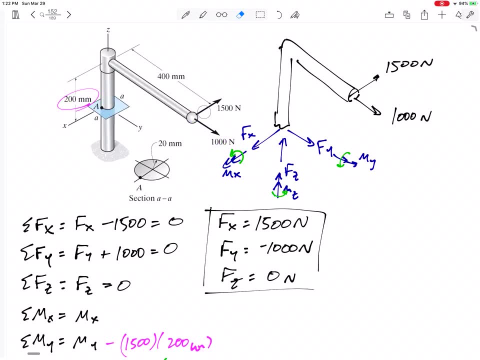 millimeters in the negative y moment. All right, can you visualize that? All right, and so that is. those are the two moments that my 1,500 newton force could cause, could create. All right, how about this 100, 1,000 newton force? How about this 1,000 newton force? right here I'll. 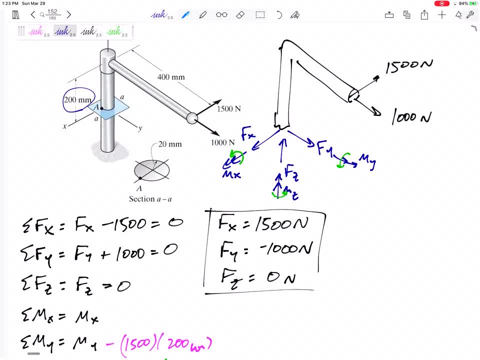 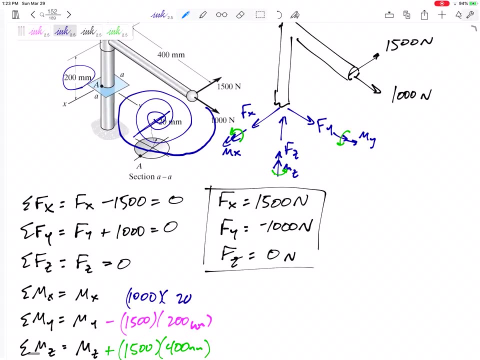 draw it in blue: 1,000 is 200 millimeters above, and so it would kind of bend down this way. It would bend down this way about the x-axis: 1,000 newtons, 200 millimeters. The force is in. 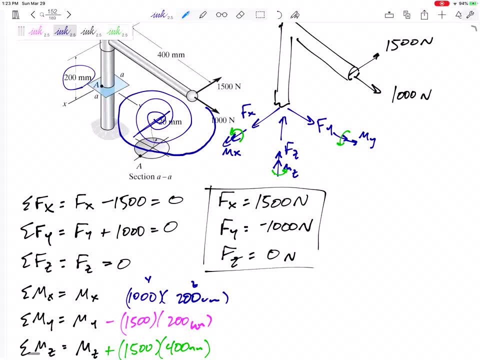 the y, the moment Arm is in the z. So yeah, an x moment, positive or negative. Bend your four fingers, curl them around. My thumb is pointed in back, this way, back this way. the negative x direction. Okay, 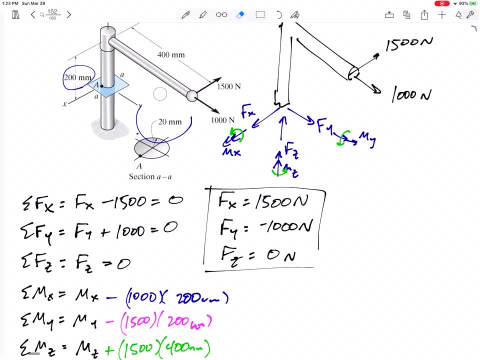 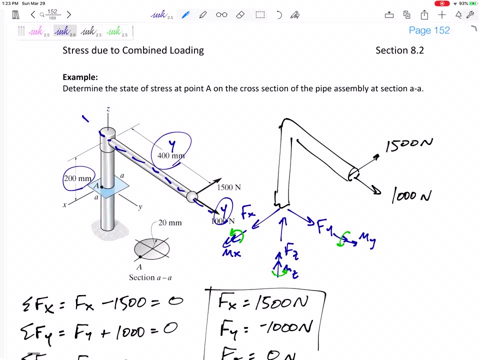 now it. that is the only moment that that 1,000 newton force would create. It is in the y direction. So this y displacement doesn't matter. This y is is not a moment. the moment arm and the force cannot not be in the same direction. 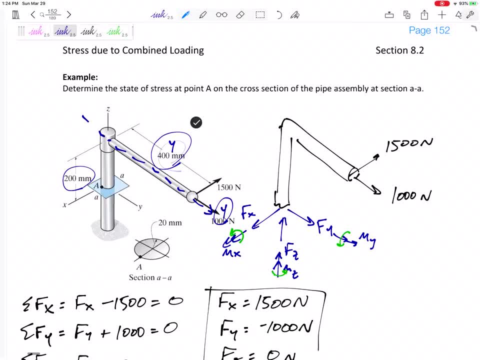 right, It doesn't really matter that it was 400 millimeters over this way. Let's see, It's a y direction that has a z moment arm. It could have had an x. So so if this 100, 1,000 newton force- sorry- was back back here behind the y z plane or in front, 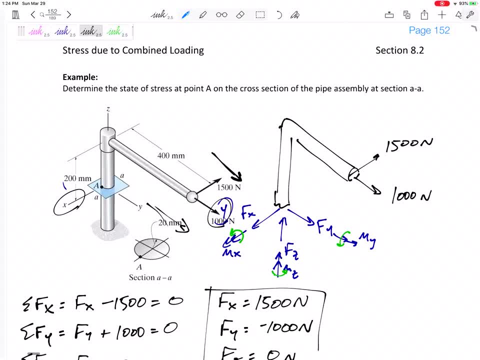 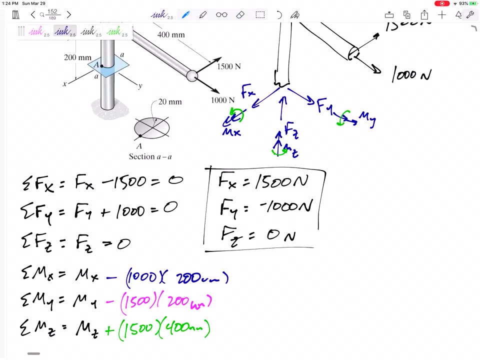 of the y z plane, then it it could have created a z moment, but it isn't. it is right on, there's no moment arm in the x direction, So that force only creates one moment. okay, So there. 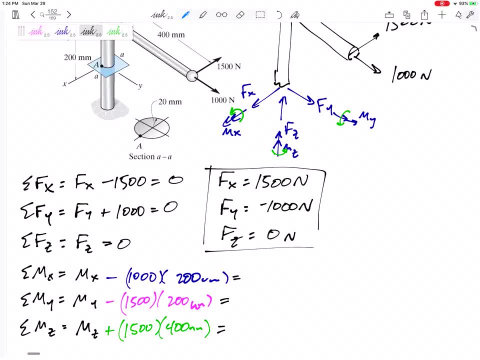 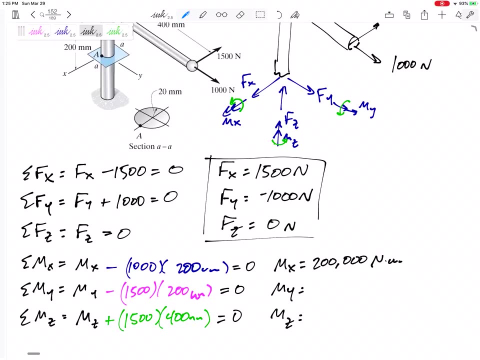 there we go. Those were all the forces creating all that we could find. Set these equal to 0.. And we would get Mx. My MZ. I've got MX 200,000 Newton millimeters, MY 300,000 Newton millimeters, MZ, negative 600,000. 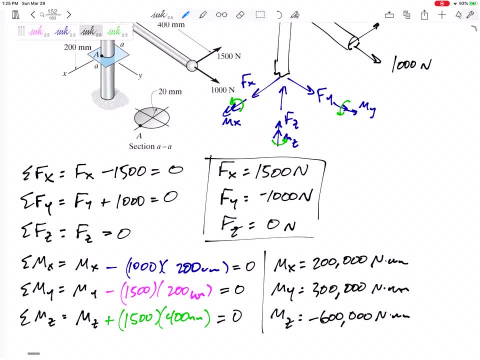 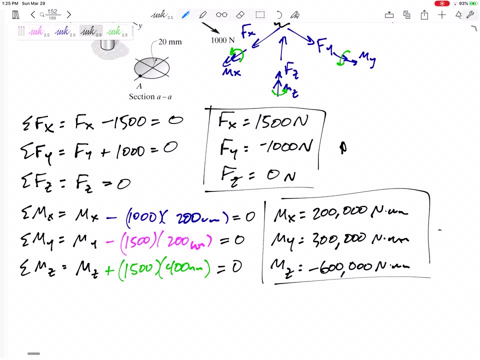 Newton millimeters. box those in because that it's so important. all right did. are you following me there? that might take some review, so I'm getting used to, but these are the internal forces, these are the internal moments at the cut. okay, so now, each of those forces and each of those moments. 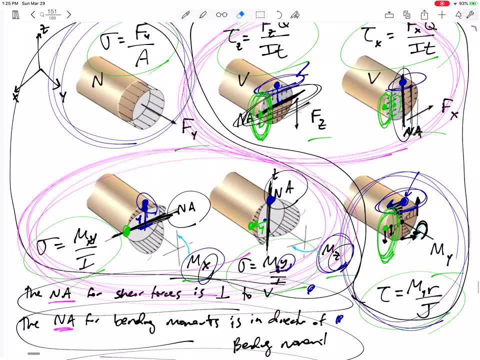 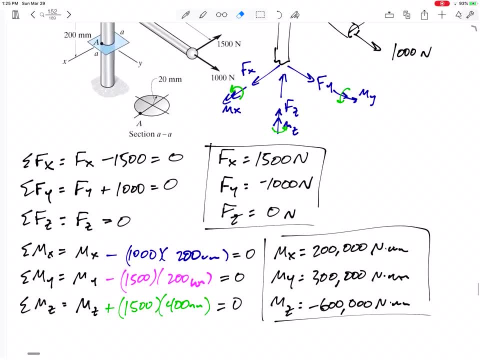 can create a different stress. when we go back to this page, you know we've got six different forces and moments creating six different types of stresses. I like to start with the axial, the one that is perpendicular to the cut right, the one that is perpendicular to the cut, this one right here and this one right here. these 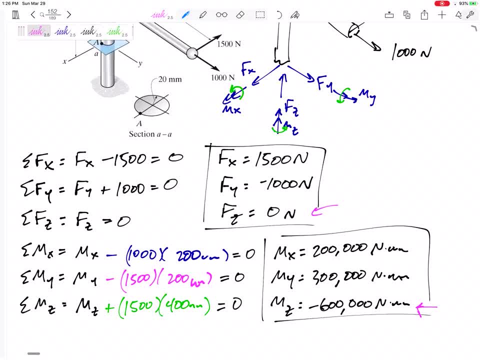 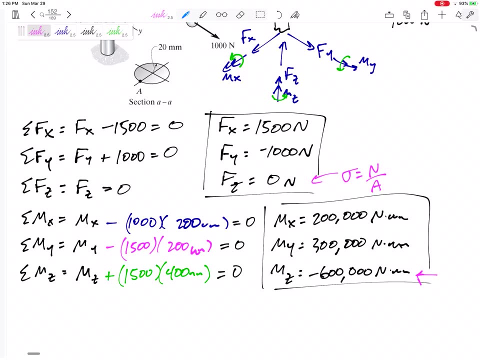 are my axial, Z is my axial direction right and FZ. the axial force would be the normal force, would be the normal stress in over a. of course it's zero, this one, we don't have to worry about that, but this one would be in over a. so then the others, the others. 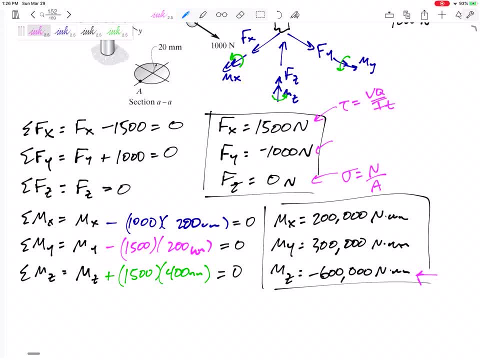 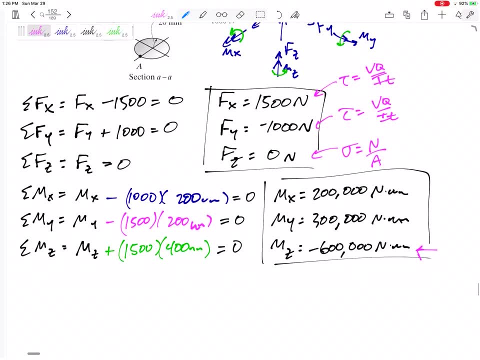 would be the VQ over IT, the shear stress VQ over IT. all right now, the moment my axial moment is is my torsional moment. it's the twisting moment. this would be the tau is TR over J, whereas the others would be the bending moments: MY over I, MY over I. 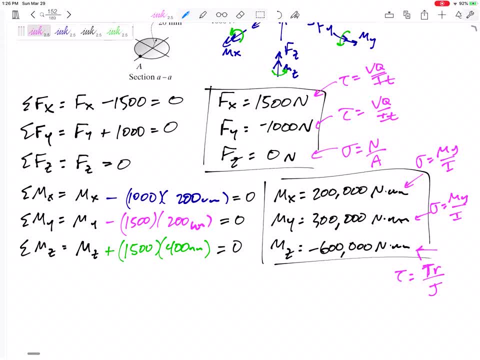 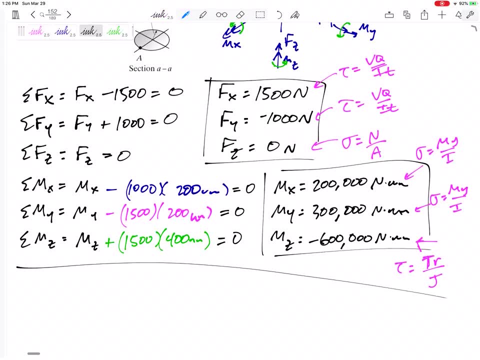 so I like to you know, just remind myself, identify what type of stress does each of them cause? all right, so now I like to do this very methodically. now let me start with this FX of 1500 Newton's. it could cause, and I say, could you know it might. 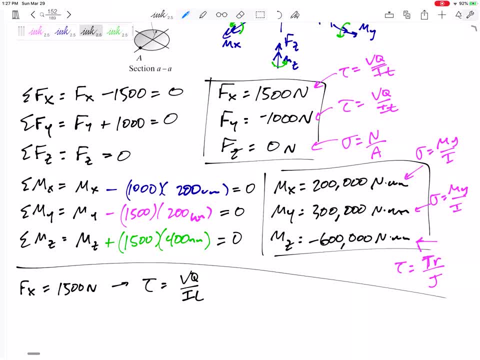 be zero, depending on the point that we're looking at, could cause VQ over IT. VQ over IT could cause V four times above. five times above and then two times over time will mean V menos a spirit. the V would be fifteen percent variance. it could now be zero, depending on the point that we're looking at. customer, call each other into any weil that you found in anyya will help you out. You can have all pleasant sounds of that which is a potential problem over time. 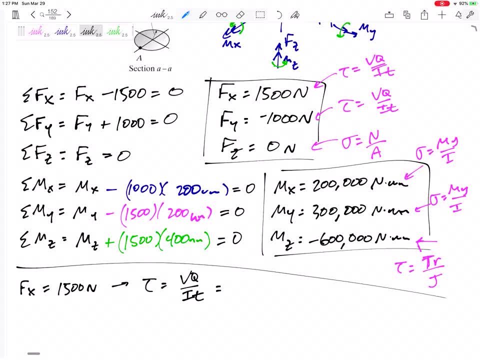 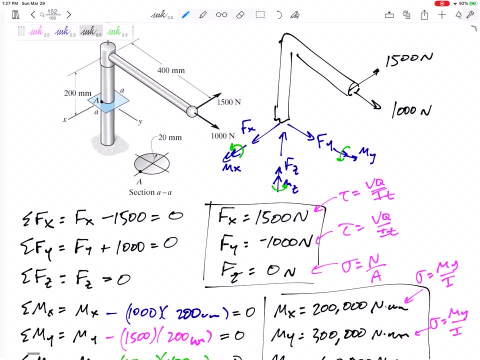 1500, but the Q we'll look at, we'll talk about All right. So I have an internal 1500 Newton force in the positive X direction, internal 1500 Newton force right here, 1500 Newtons in the X direction. It creates a shear. So there's point A that I'm looking at. It creates a shear. 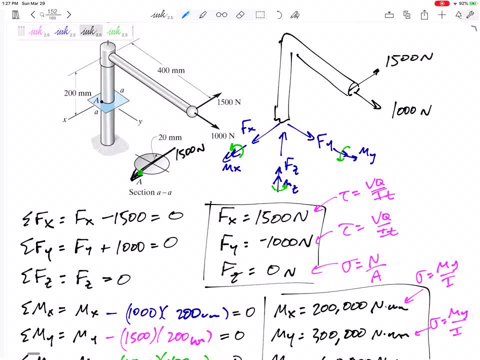 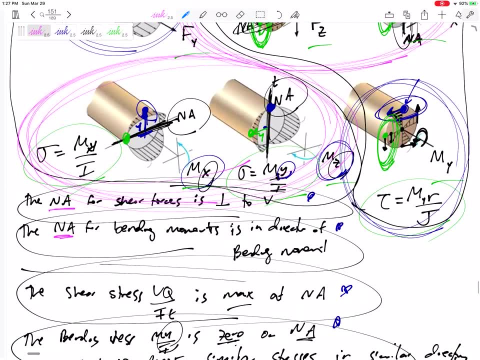 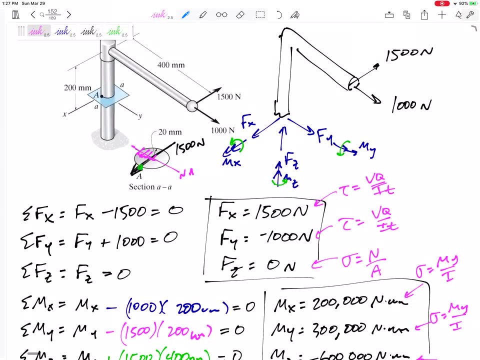 stress distribution. that would look like this. So, first of all, where's the neutral axis? The neutral axis is perpendicular to the shear force, So let's remember about this. The neutral axis for shear stress is perpendicular to B, And it would be largest if we were looking at a point on the 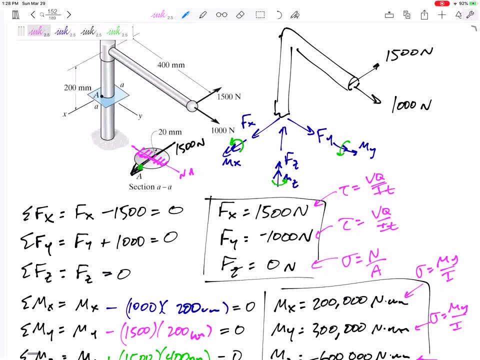 neutral axis, then that would be the largest. I would do VQ over IT. The Q would be Y prime, A prime and A prime would be this: That would be A prime, But we're not looking at a point here or here or here. 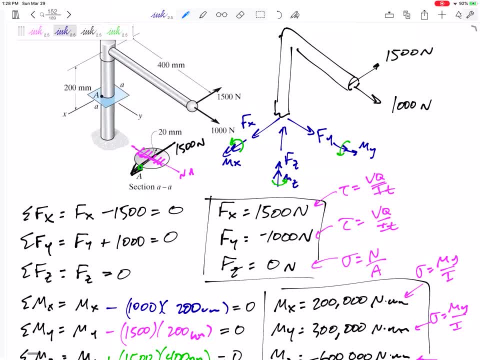 Are we? We are looking at a point right here on this leading edge, And I know that for shear stress on the very leading edge, right where it starts, right where it ends, that force, you know, I think about that force as kind of beginning on this leading edge, ending on the 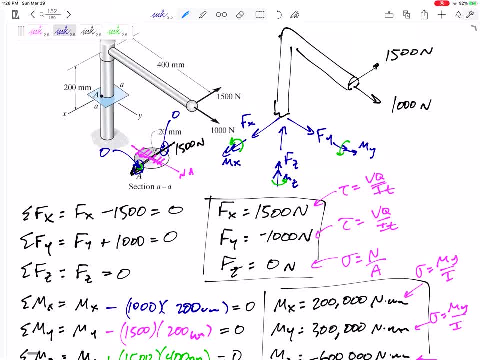 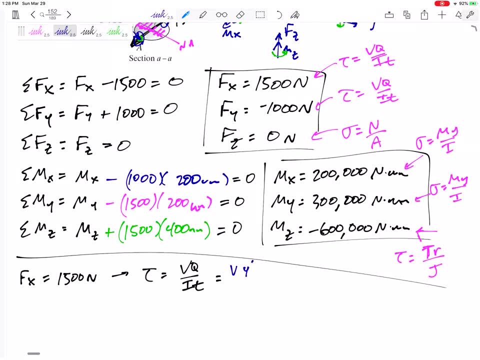 trailing edge. It is zero. It is zero right here. You know, if you really wanted to think about this zero right here, You would do the V, the Q is Y prime, A prime, And that A prime, which is the area away from neutral. 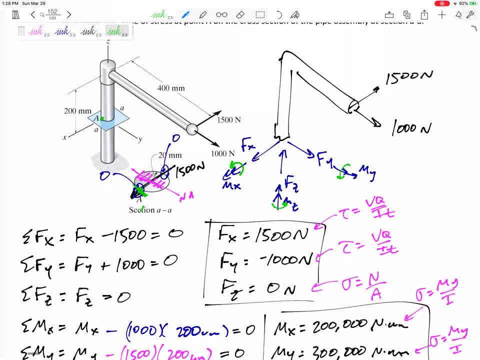 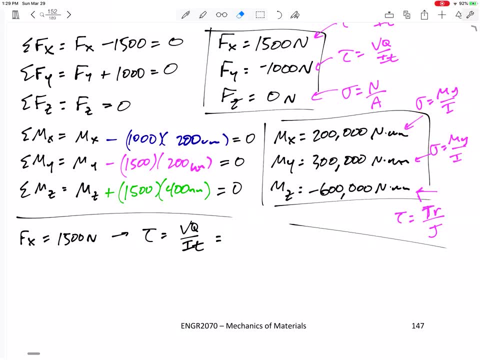 axis. if you're already out here on the edge, there's nothing away from the neutral axis anymore. That A prime is zero, All right. so this is zero because of point A. because of the point All right, it does have a V of 1,500, but at point A the shear stress is zero. 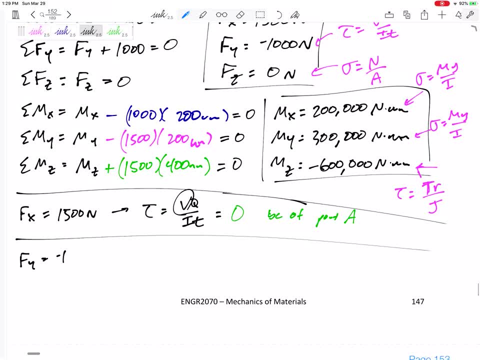 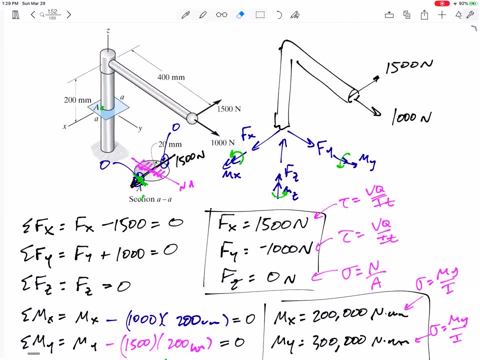 All right, let's look at FY. FY negative 1,000.. It's a shear. It could be VQ over IT. Let me erase this, because I have a new neutral axis. I've got a new force that I'm looking at. Don't reuse any of that, All right. so now I 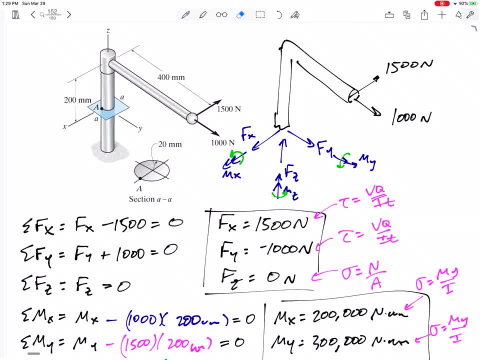 have a force of in the negative Y direction of 1,000 newtons. What would that look like? I've got a force right here, right here, of 1,000 newtons, right there. Where's my neutral axis? Neutral axis is: 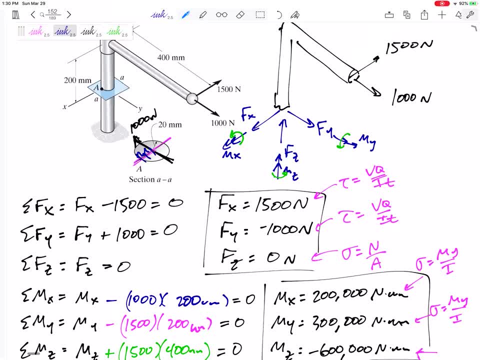 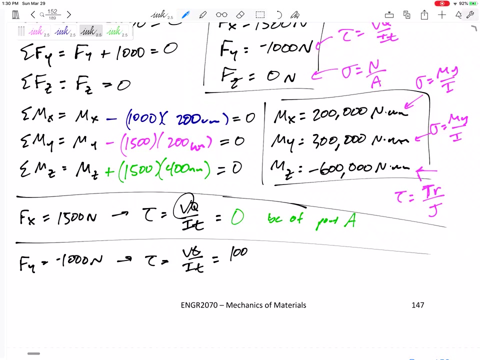 right here Shear VQ over IT would be largest. at a maximum It would be zero right here and right here. And so point A is on the neutral axis and it's going to be one of the larger points of shear due to that 1,000 newton force. So let's do the VQ over IT. So this would be V 1,000. 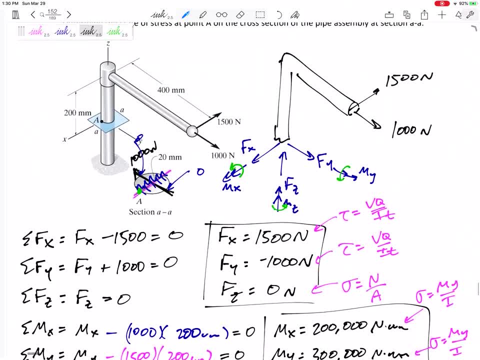 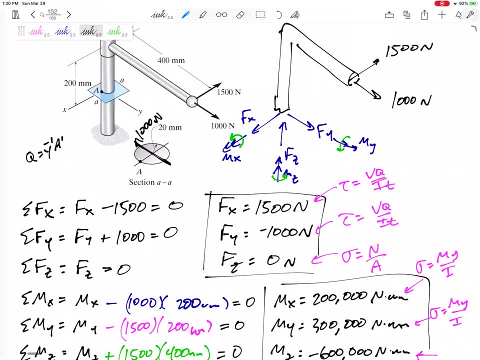 newtons. Q, all right, Q is Y prime A prime, Q is Y prime A prime. Let me draw this: 1,000 newtons. Q is Y bar prime, A prime, A prime. I'll start with A prime, because it's easiest. It's the 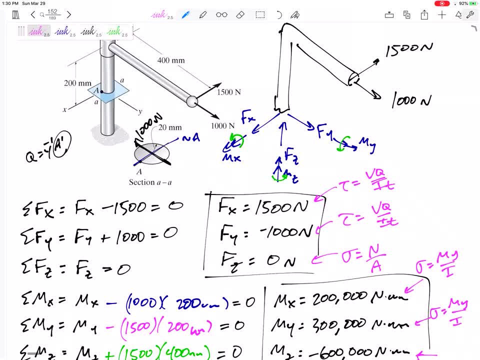 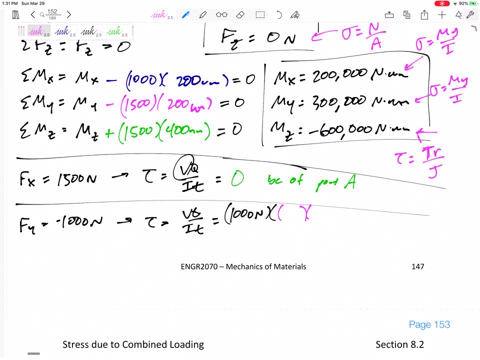 area. here's the neutral axis. It's the area away from the neutral axis of the point I'm interested in. That right there would be A prime. That right there would be A prime. Let me go ahead and do that. What's that area? The radius is F20.. The area would be half of pi R squared. 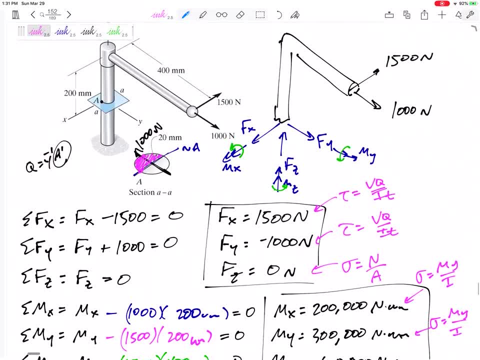 All right. and then the Y bar prime is the distance from the neutral axis to the centroid of A prime. So that distance right there, from here to there, that length right there, look on your formula sheet: The centroid of a half circle, the location of its 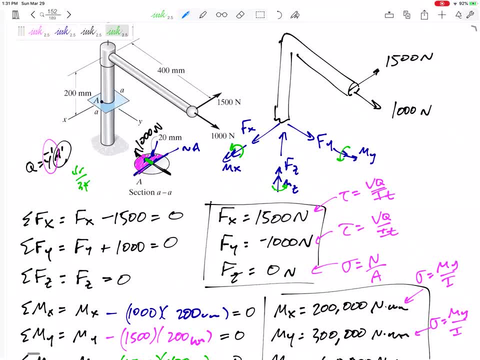 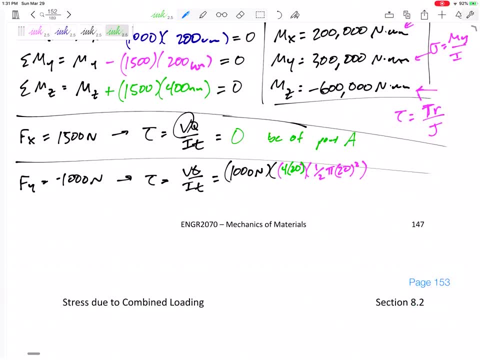 centroid is 4R over 3 pi, And so that is that green line: 4R over 3 pi. This would be 4R over 3 pi right there. That was the Q. That was a tough one, but not too bad. 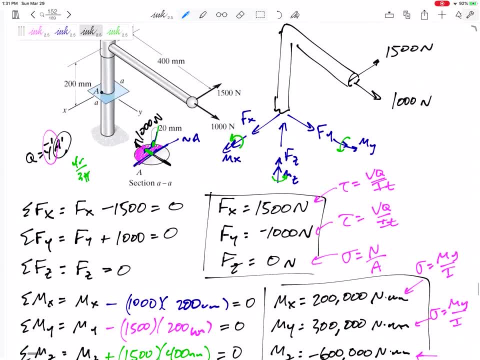 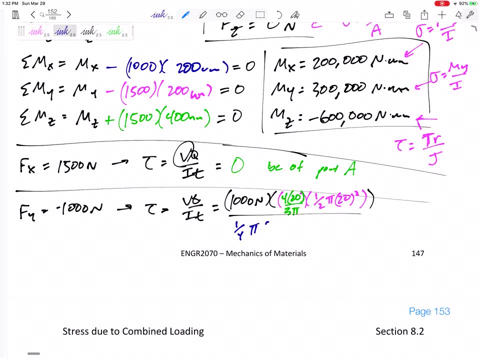 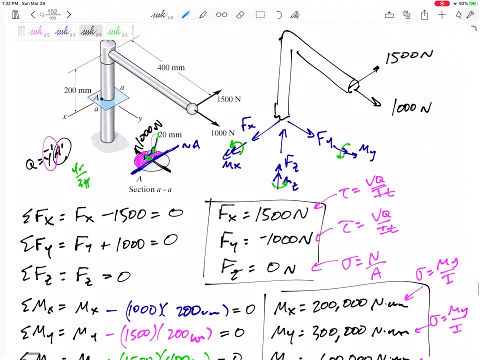 All right, so that's the V, the Q, The I. would be the I about the neutral axis On that formula sheet. look at a circle. What is the I for this circular shape? One-fourth pi R to the fourth, All right, and then what is the thickness, at the point that I'm interested in The thickness? 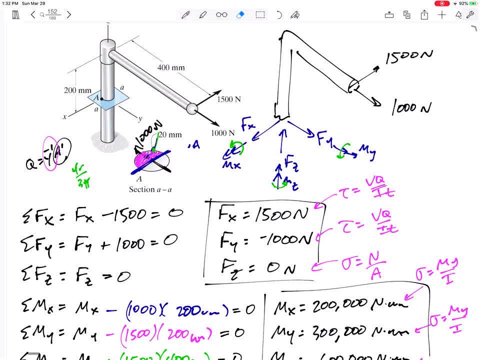 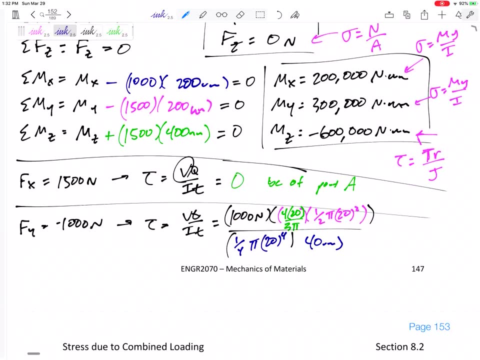 right here the thickness. sorry, it's going to be perpendicular to this V. All right, this V is right here. So the thickness would be this distance, right here the diameter. The thickness would be the diameter: 40 millimeters. I think everything was in millimeters, millimeters. 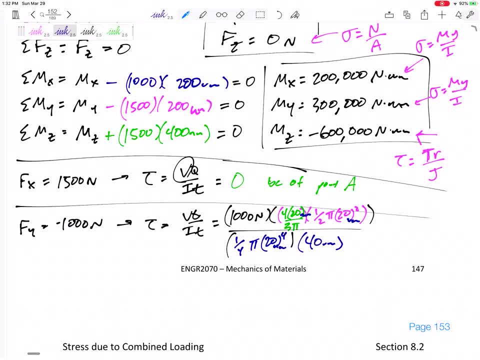 millimeters Now. so I'm left with Newton's over millimeter squared, which is MPa. This would be 1.061 MPa. That would be a tau. Specify whether it's a tau or a sigma. This is a tau. this is a shear stress, And let's say what direction this is in. Let's specify. 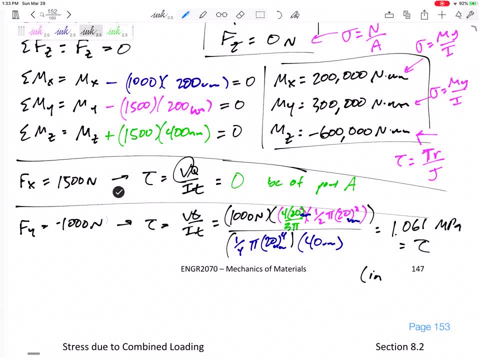 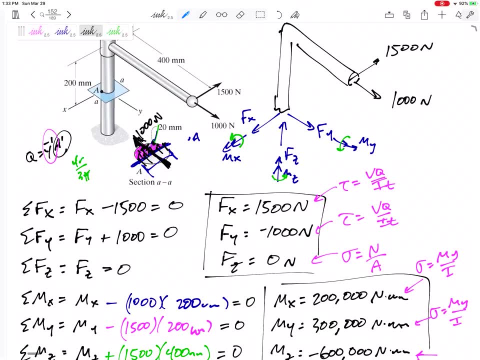 what direction this is in. Well, whatever direction the force was in, that's the direction all of these shear arrows are going to be in. 007②No matter what direction I went in, they were in a new direction, No matter where. 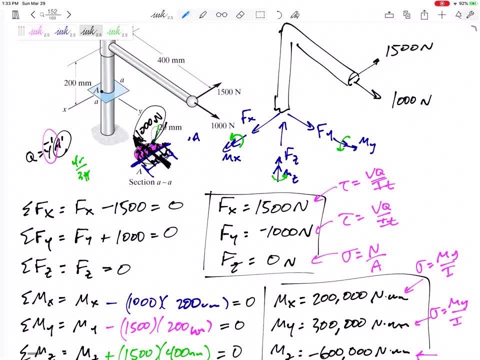 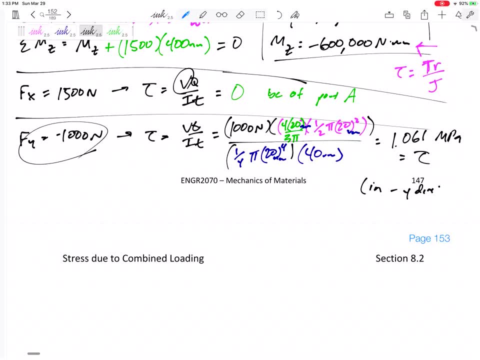 I am. those arrows are going to be in a new direction, No matter what direction I went in. that force of negative 1,000 or 1,000 in the negative y direction, this shear stress is in the negative y direction. 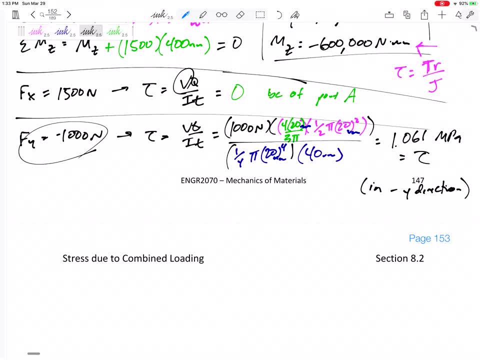 I'm going to specify that because I might want to combine this with some other shear stresses that I've calculated. I might want to combine that with some other ones. I need to make sure they're the same type of stress in the same direction. 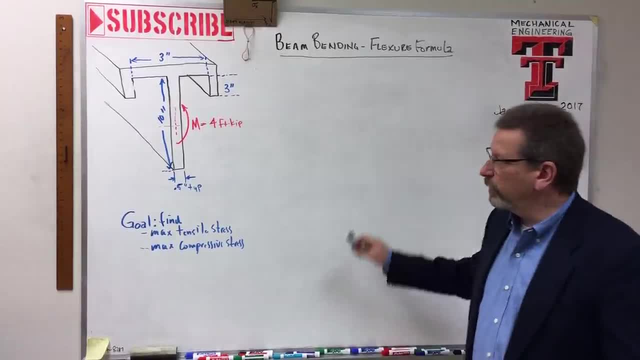 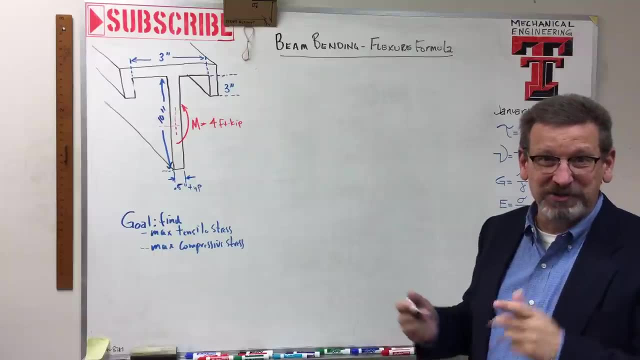 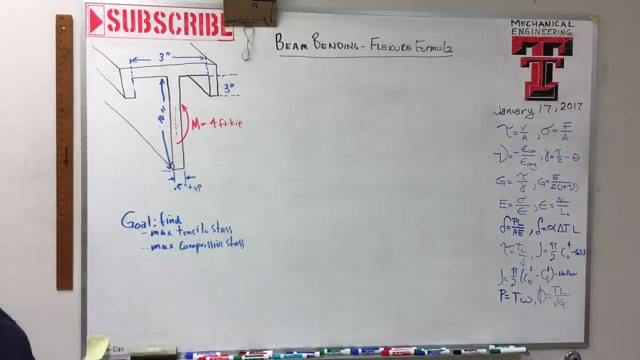 Okay, team, welcome back. We're going to talk today about the beam bending. flex your formula. We're going to get a new formula on our formula sheet today, Woohoo, Okay. so what we're talking today about is beam bending. Okay, so if I have my beam, here's my beam again. right, my nerf noodle. 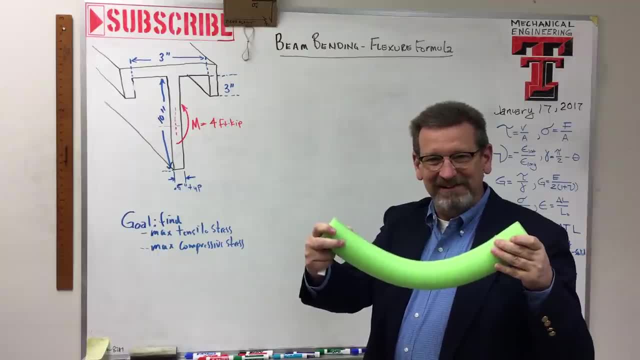 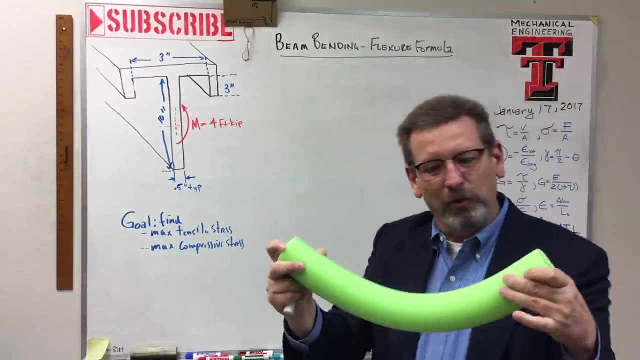 right as I start bending this beam. what's happening to that beam? Well, if you can see the top of my beam- I don't know if you can see that or not, but there's little wrinkles on it, right. Why are there wrinkles on the top? Because, as I bend this, the top fibers of this beam are 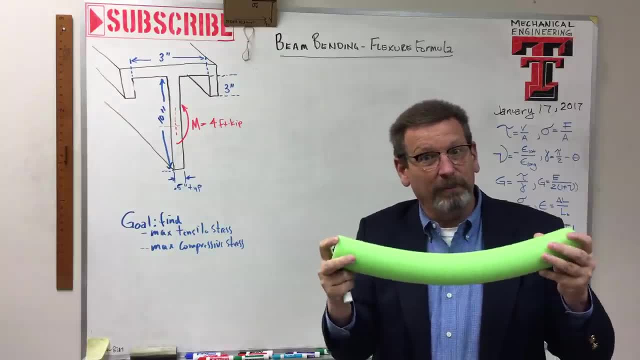 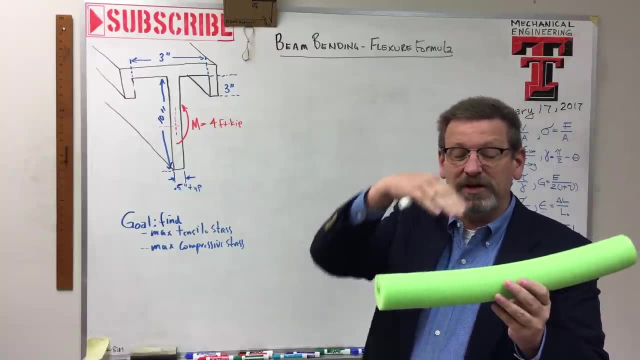 in compression right, Whereas the bottom ones down here are being stretched. they're in tension. So somewhere in between the top and the bottom, there has to be something going on. It has to switch from compression to tension right. Well, it does that at what's called the neutral axis. 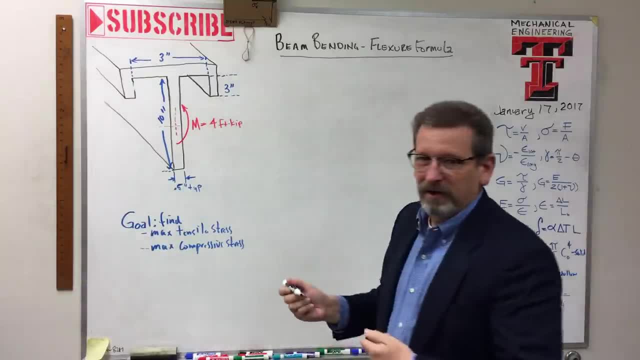 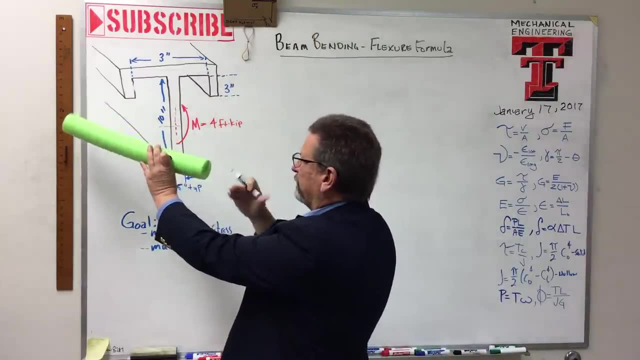 okay, or the centroidal axis Of the part. Here's a beam I have that. I have a cross-section of right. The beam goes into the board like that and I'm taking a cross-section and the end of it. look at that cross-sectional. 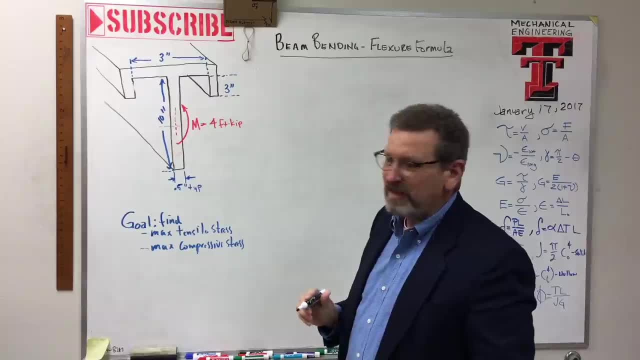 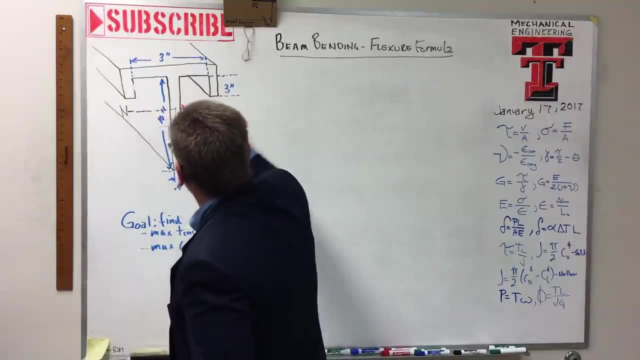 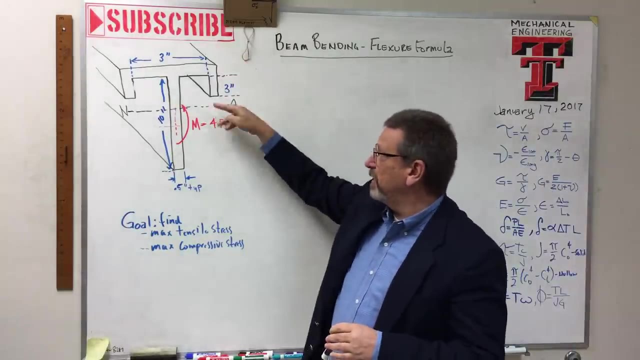 view is kind of a T-shaped okay. So somewhere on this thing, this beam is what's called the neutral axis. right, The neutral axis. So if it's compression at the top and tension at the bottom, what's going on with the neutral axis?